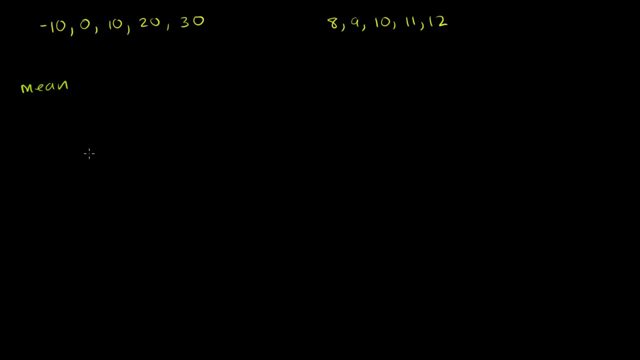 But if you are going to go further in statistics, I just want to make that clarification. Now, the population mean or the arithmetic mean of this data set right here, it is negative. 10 plus 0 plus 10 plus 20 plus 30 over, we have 5 data points. 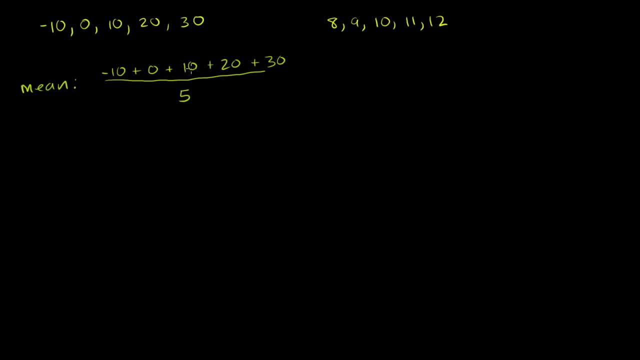 over 5.. And what is this? equal to? That? negative 10 cancels out with that 10.. 20 plus 30 is 50 divided by 5.. It's equal to 10.. Now, what's the mean of this data set? 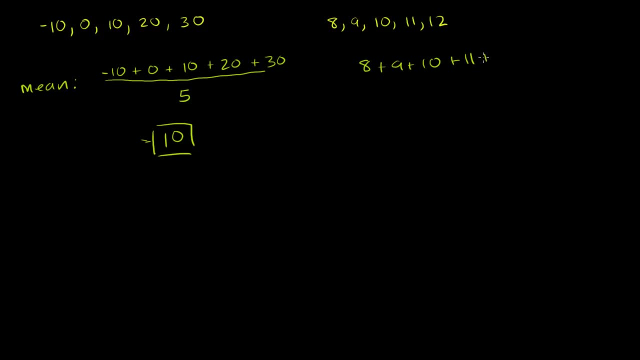 8 plus 9 plus 10 plus 11 plus 12.. All of that over 5.. And the way we could think about it, 8 plus 12 is 20.. 9 plus 11 is another 20.. So that's 40.. 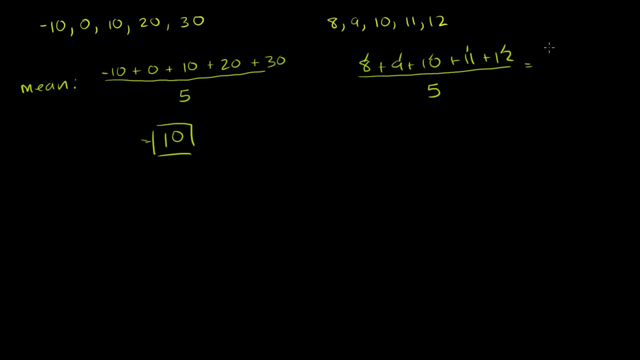 And then we have a 50 there, Add another 10. So this is once again going to be 50 over 5.. So this has the exact same population means, Or, if you don't want to worry about the word population or, 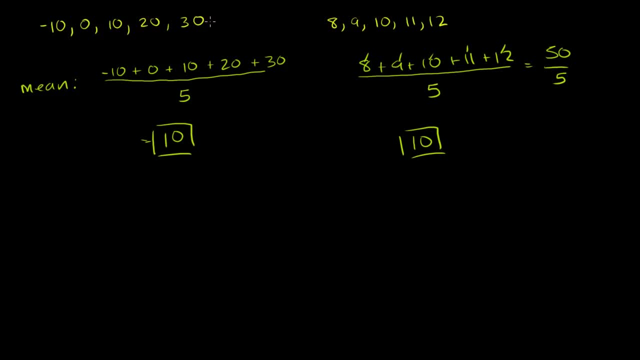 sample and all of that. both of these data sets have the exact same arithmetic mean. When you average all these numbers and divide by 5, or when you take the sum of these numbers divide by 5,, you get 10.. Sum of these numbers divided by 5,, you get 10 as well. 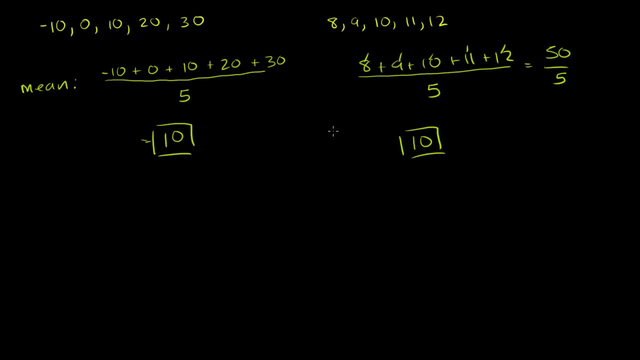 But clearly these sets of numbers are different. If you just looked at this number, you'd say, oh, maybe these sets are very similar to each other. But when you look at these two data sets, one thing might pop out at you. 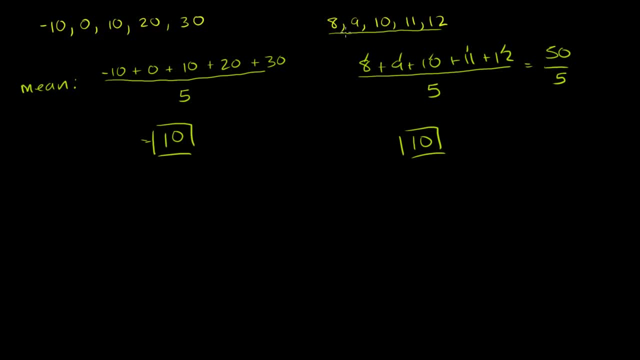 All of these numbers are very close to 10.. I mean, the furthest number here is 2 away from 10.. 12 is only 2 away from 10.. Here these numbers are further away from 10. Even the closer ones are still 10 away. and then these: 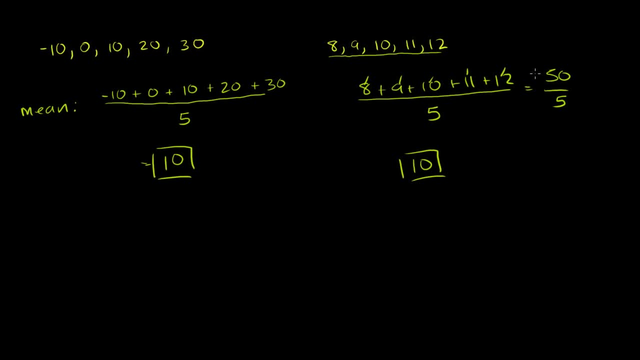 guys are 20 away from 10.. So this right here, this data set right here, is more disperse right. These guys are further away from our mean than these guys are from this mean. So let's think about different ways we can measure dispersion. 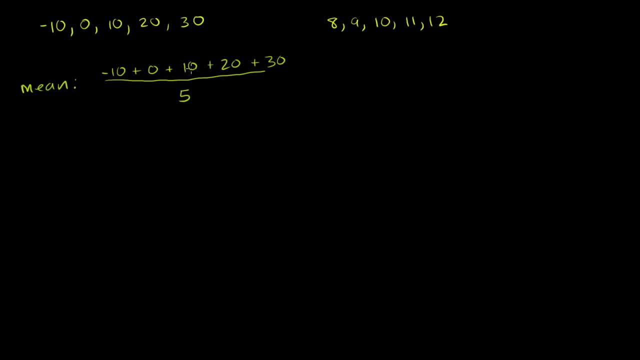 over 5.. And what is this? equal to? That? negative 10 cancels out with that 10.. 20 plus 30 is 50 divided by 5.. It's equal to 10.. Now, what's the mean of this data set? 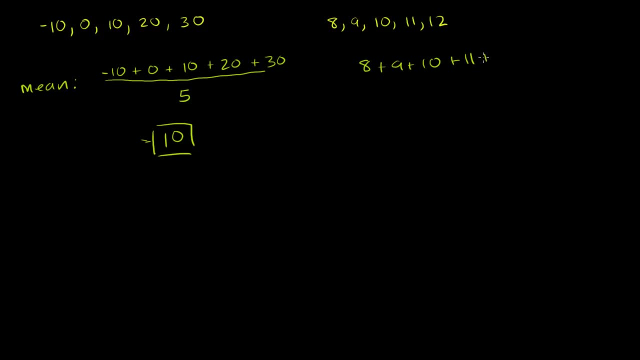 8 plus 9 plus 10 plus 11 plus 12.. All of that over 5.. And the way we could think about it, 8 plus 12 is 20.. 9 plus 11 is another 20.. So that's 40.. 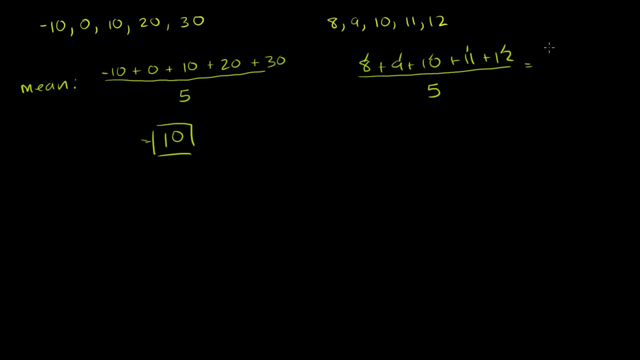 And then we have a 50 there, add another 10. So this is, once again, is going to be 50 over 5.. So this has the exact same population means, Or, if you don't want to worry about the word population or, 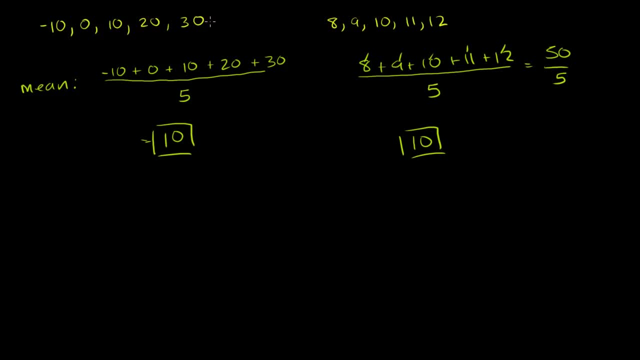 sample and all of that. both of these data sets have the exact same arithmetic mean. When you average all these numbers and divide by 5, or when you take the sum of these numbers divide by 5,, you get 10.. Sum of these numbers divided by 5,, you get 10 as well. 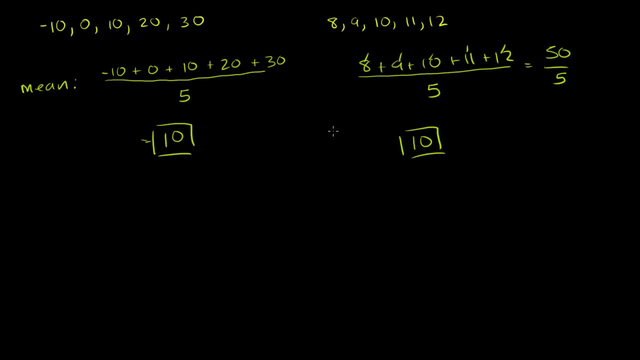 But clearly these sets of numbers are different. If you just looked at this number, you'd say, oh, maybe these sets are very similar to each other. But when you look at these two data sets, one thing might pop out at you. 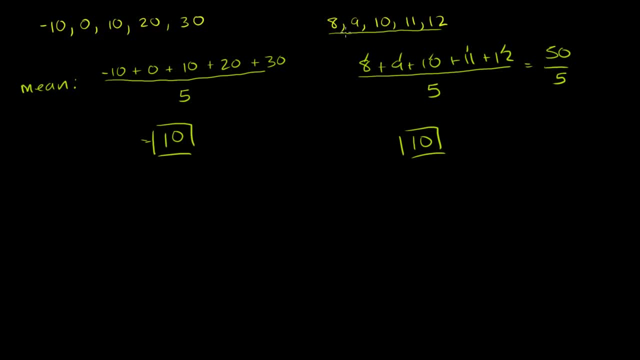 All of these numbers are very close to 10.. I mean, the furthest number here is 2 away from 10.. 12 is only 2 away from 10.. Here these numbers are further away from 10. Even the closer ones are still 10 away. and then these: 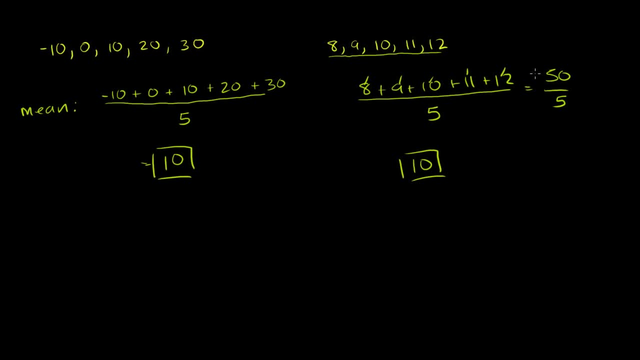 guys are 20 away from 10.. So this right here, this data set right here, is more disperse right. These guys are further away from our mean than these guys are from this mean. So let's think about different ways we can measure dispersion. 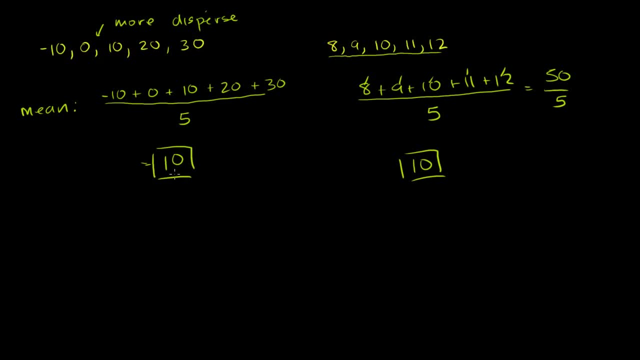 or how far away we are from the center on average. Now, one way- this is kind of the most simple way- is the range, And you won't see it used too often, but it's kind of a very simple way of understanding how far is the spread between 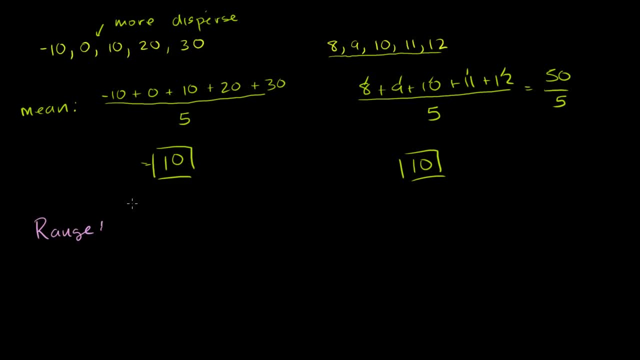 the largest and the smallest number. And literally you take the largest number, which is 30 in our example, and from that you subtract the smallest number, so 30 minus negative 10, which is equal to 40, which tells us that the difference between the 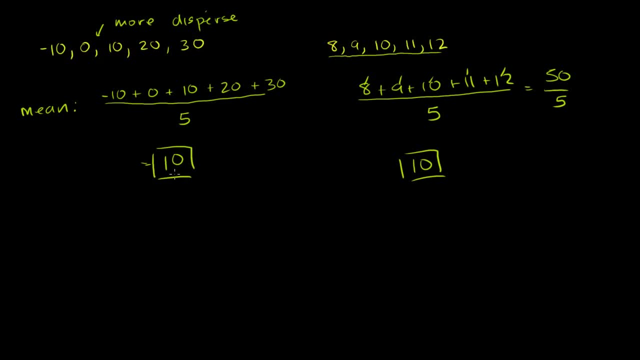 or how far away we are from the center on average. Now, one way- this is kind of the most simple way- is the range, And you won't see it used too often, but it's kind of a very simple way of understanding how far is the spread between 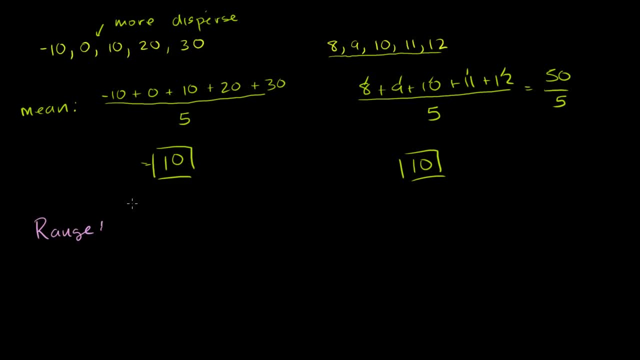 the largest and the smallest number. And literally you take the largest number, which is 30 in our example, and from that you subtract the smallest number, so 30 minus negative 10, which is equal to 40, which tells us that the difference between the 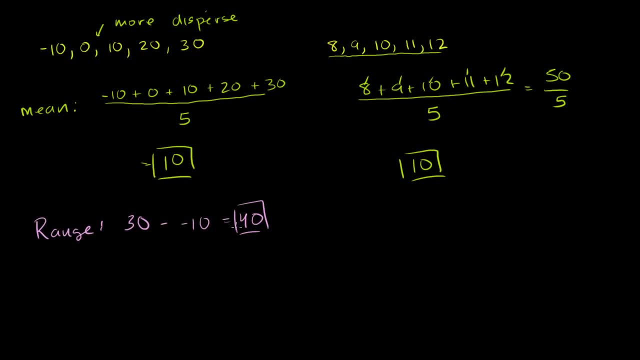 largest and the smallest number is 40. So we have a range of 40 for this data set. Here the range is the largest number, 12.. Minus the smallest number, which is 8,, which is equal to 4.. 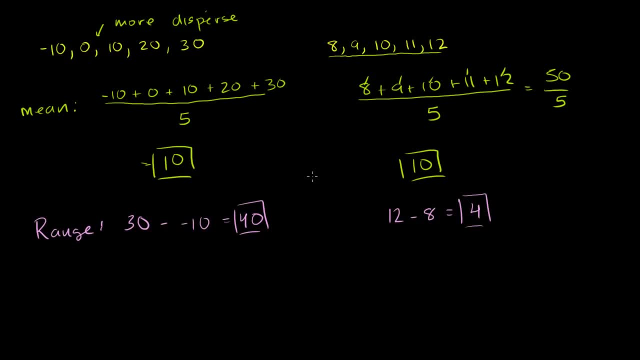 So here range is actually a pretty good measure of dispersion. We say, OK, both of these guys have a mean of 10. But when I look at the range, this guy has a much larger range. so that tells me this is a more disperse set. 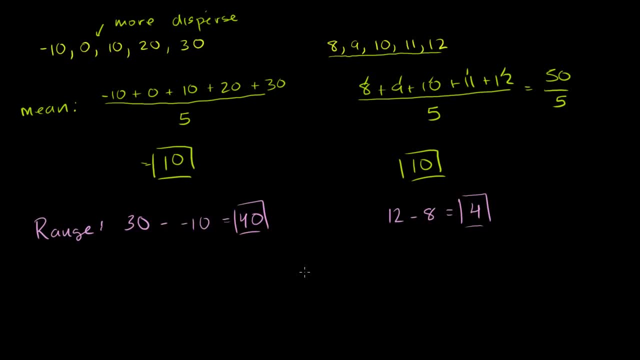 But range is always not going to tell you the whole picture. You might have two data sets with the exact same range where still, based on how things are bunched up, it could still have very little dispersion. So you might have two data sets with the exact same range. 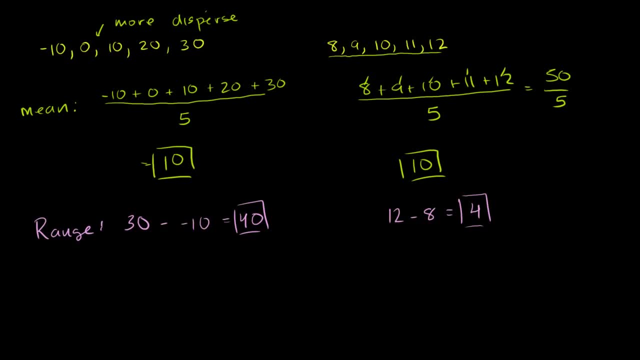 where still, based on how things are bunched up, it could still have very little dispersion. All right, So we're going to use a very different distribution of where the numbers lie. Now, the one that you'll see used most often is called the. 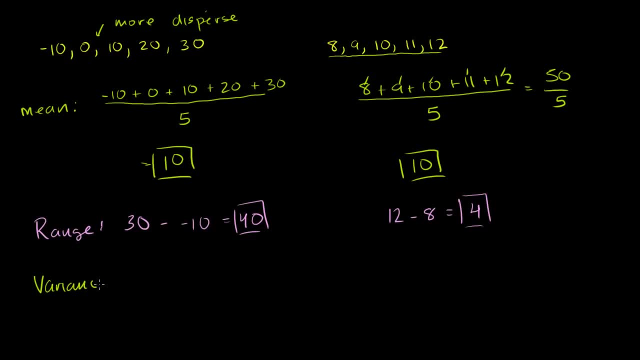 variance. Actually, you're going to see the standard deviation in this video. That's probably what's used most often, But it has a very close relationship to the variance. So the symbol for the variance and we're going to deal with the population variance. 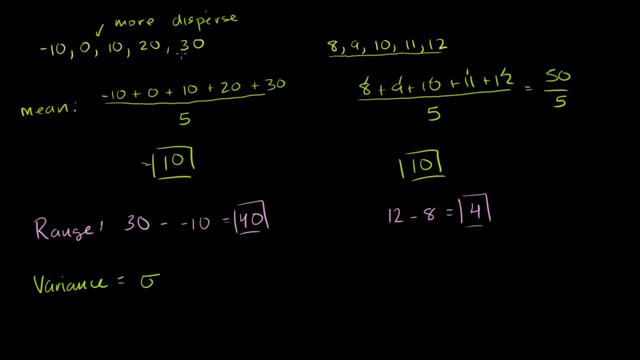 Once again, we're assuming that this is all of the data for our whole population, that we're not just sampling, taking a subset of the data. So the variance is a very large number here. Its symbol is literally this sigma, this Greek letter squared. 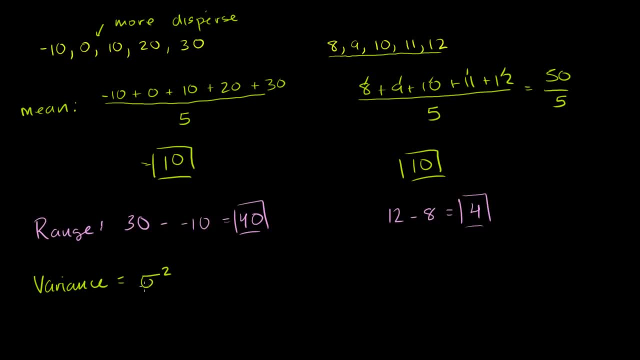 That is the symbol for variance And we'll see that the sigma letter actually is the symbol for standard deviation, And that is for a reason. But anyway, the definition of variance is: you literally take each of these data points, find the difference between: 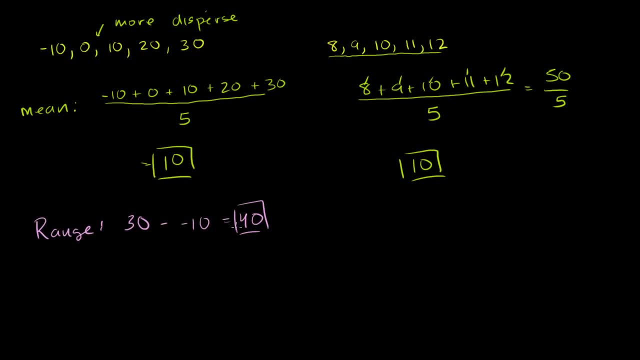 largest and the smallest number is 40. So we have a range of 40 for this data set. Here the range is the largest number, 12.. Minus the smallest number, which is 8,, which is equal to 4.. 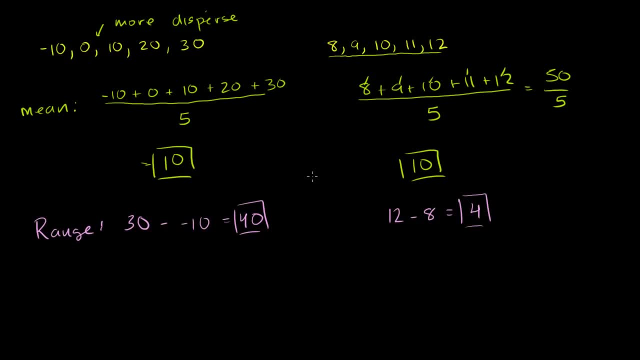 So here range is actually a pretty good measure of dispersion. We say, OK, both of these guys have a mean of 10. But when I look at the range, this guy has a much larger range. so that tells me this is a more disperse set. 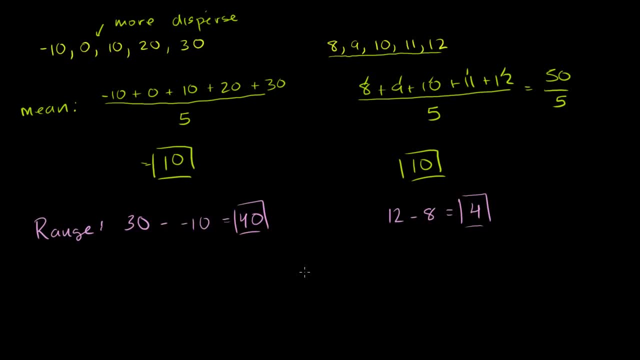 But range is always not going to tell you the whole picture. You might have two data sets with the exact same range where still, based on how things are bunched up, it could still have very little dispersion. So you might have two data sets with the exact same range. 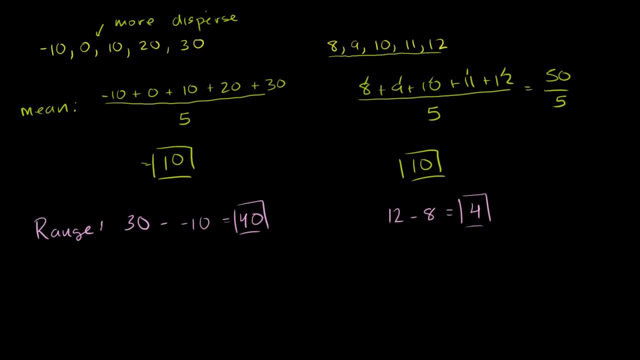 where, still, based on how things are bunched up, it could still have very little dispersion. So you might have two data sets with the exact same range, which is very different distributions of where the numbers lie. Now the one that you'll see used most often is called the 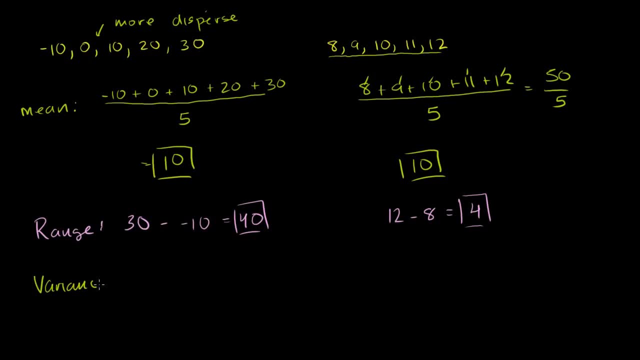 variance. Actually, you're going to see the standard deviation in this video. That's probably what's used most often, But it has a very close relationship to the variance. So the symbol for the variance and we're going to deal with the population variance. 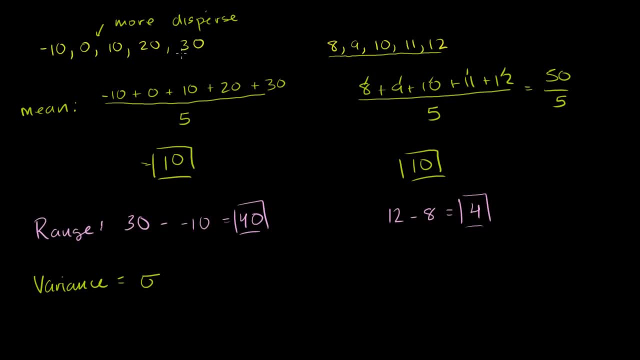 Once again, we're assuming that this is all of the data for our whole population, that we're not just sampling, taking a subset of the data. So the variance Its symbol is literally this sigma, this Greek letter squared, that is the symbol for variance. 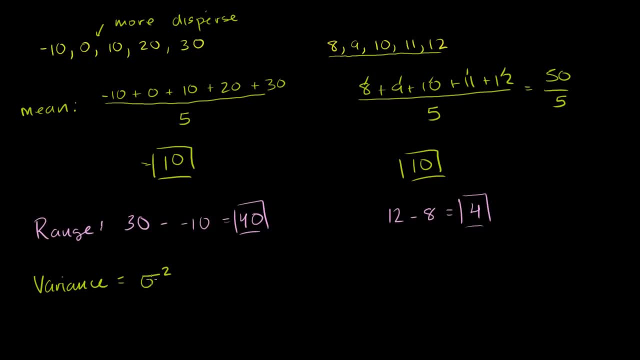 And we'll see that the sigma letter actually is the symbol for standard deviation, And that is for a reason. But anyway, the definition of variance is: you literally take each of these data points, find the difference between those data points and your mean, square them and then 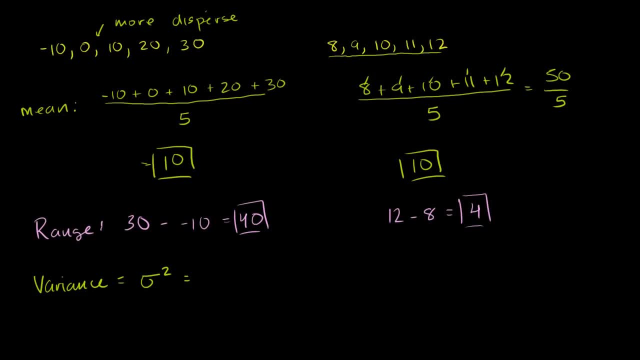 take the average of those squares. I know that sounds very complicated, But when I actually calculate it you're going to see it's not too bad. So remember, the mean here is 10.. So I take the first data point. I say it's. let me do it over here. 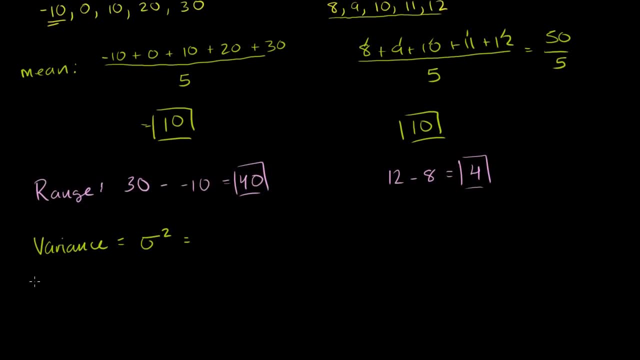 Let me scroll down a little bit. So I take the first data point, negative 10.. From that I'm going to subtract our mean And I'm going to square that. So I just found the difference from that first data point to. 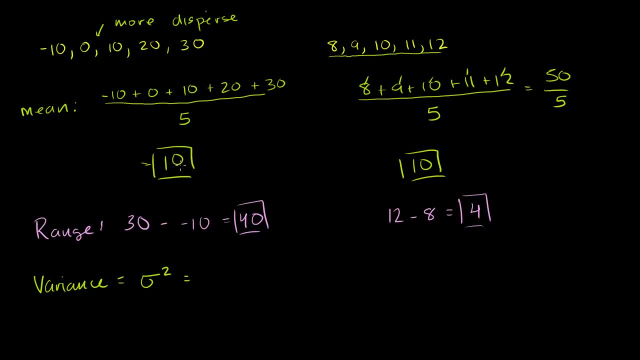 those data points and your mean, square them and then take the average of those squares. I know that sounds very complicated, but when I actually calculate it you're going to see it's not too bad. So remember, the mean here is 10.. 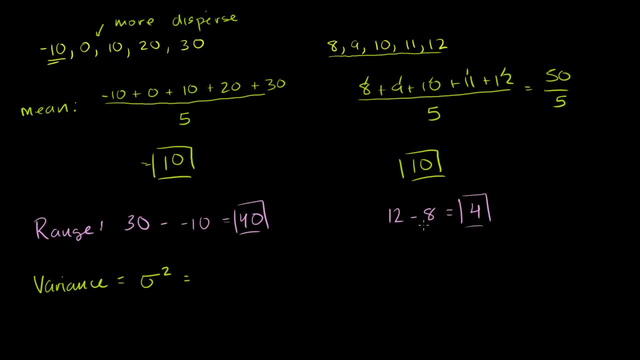 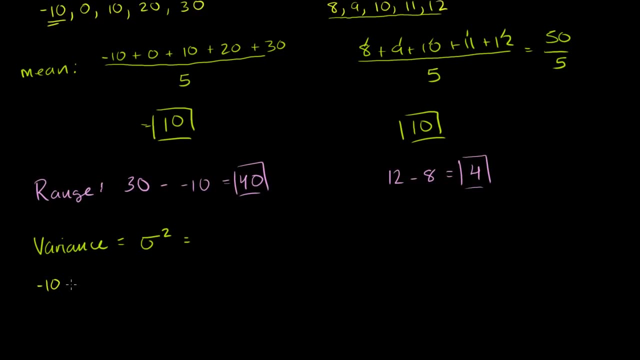 So I take the first data point. I say it's: let me do it over here, Let me scroll down a little bit. So I take the first data point: negative 10.. From that I'm going to subtract our mean and I'm 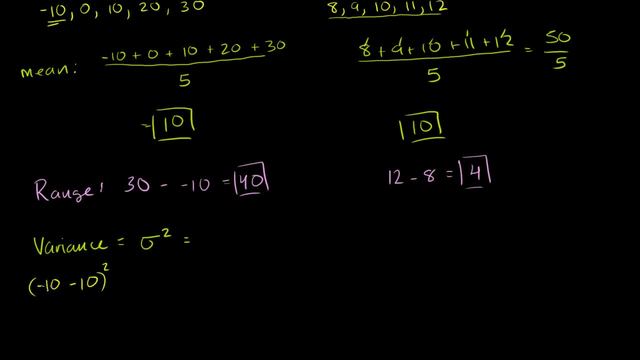 going to square that. So I just found the difference from that first data point to the mean and squared it, And that's essentially to make it positive Plus the second data point: 0 minus 10.. Minus the mean, This is the mean. 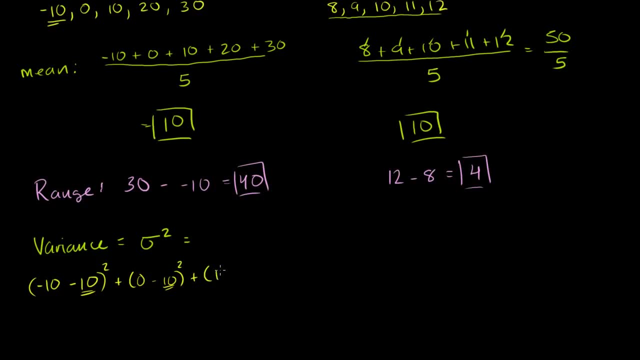 This is that 10 right there Squared Plus 10 minus 10 squared. That's the middle 10 right there Plus 20 minus 10.. That's the 20. Squared Plus 30 minus 10 squared. 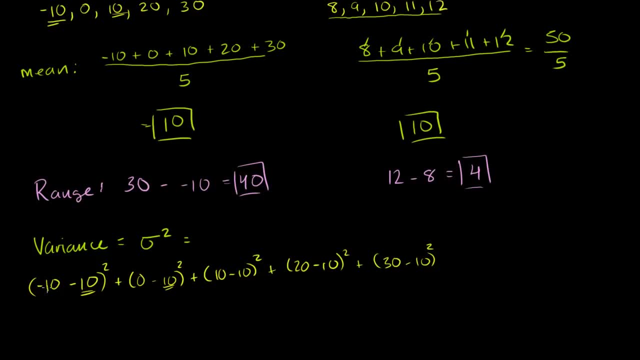 So this is the squared differences between each number and the mean. This is the mean, This is the mean. right there, That is the mean. I'm finding the difference between every data point and the mean, squaring them, summing them up and then. 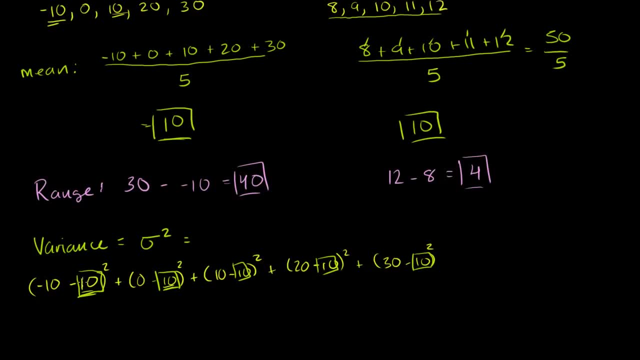 dividing by that number of data points. I'm taking the average of these numbers of the squared distances. So when you say it kind of verbally it sounds very complicated, but you're just taking each number. What's the difference between that? the mean square it. 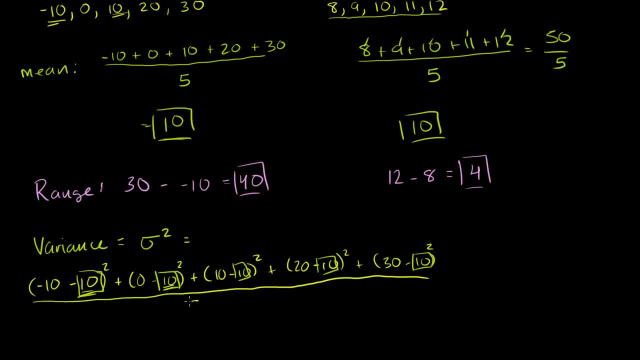 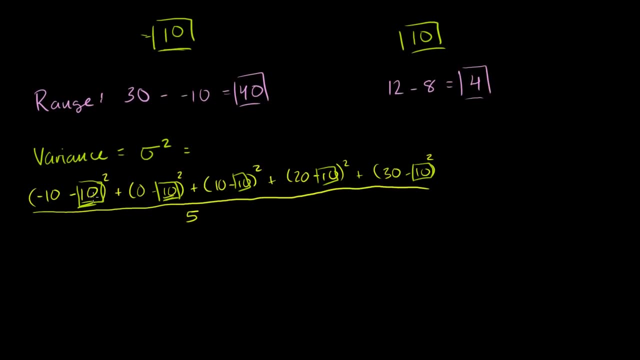 Take the average of those, So I have 1,, 2,, 3,, 4, 5.. Divide by 5.. So what is this going to be equal to? What is this going to be equal to? Negative 10 minus 10 is negative 20.. 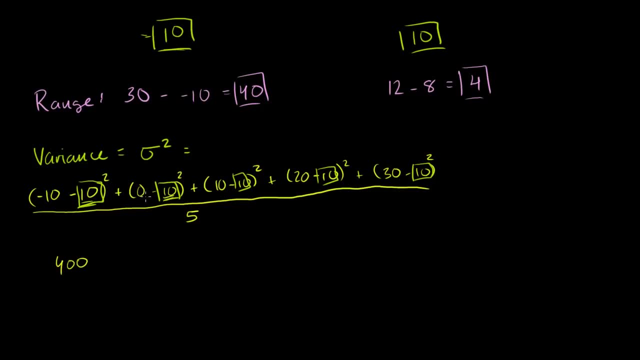 Negative: 20 squared is 400.. 0 minus 10 is negative, 10 squared is 100, so plus 100.. 10 minus 10 squared, that's just 0 squared, which is 0.. Plus 20 minus 10 is 10 squared is 100.. 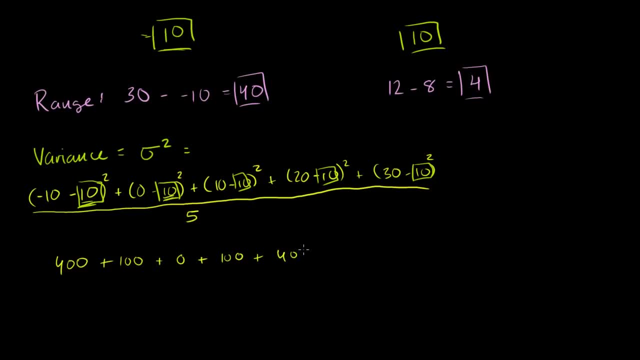 Plus 30 minus 10, which is 20, squared is 400.. All of that over 5.. And what do we have here? 400 plus 100 is 500, plus another 500 is 1,000. It's equal to 1,000 over 5, which is equal to 200.. 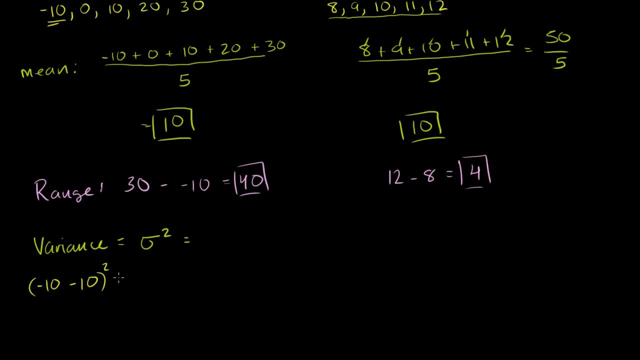 the mean and squared it, And that's essentially to make it positive. Plus the second data point: 0 minus 10 minus the mean. This is the mean, This is that 10.. Right there, Squared Plus 10 minus 10 squared. 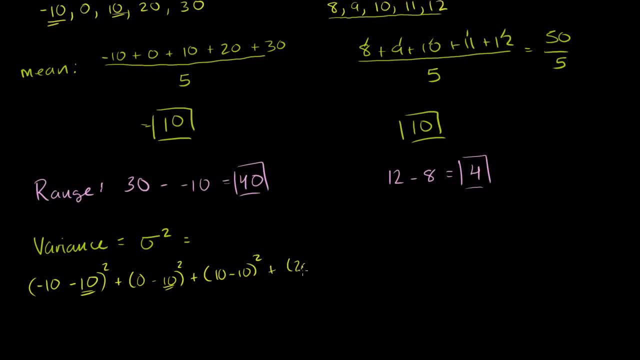 That's the middle 10 right there, Plus 20 minus 10.. That's the 20. Squared Plus 30 minus 10 squared. So this is the squared differences between each number and the mean. This is the mean. 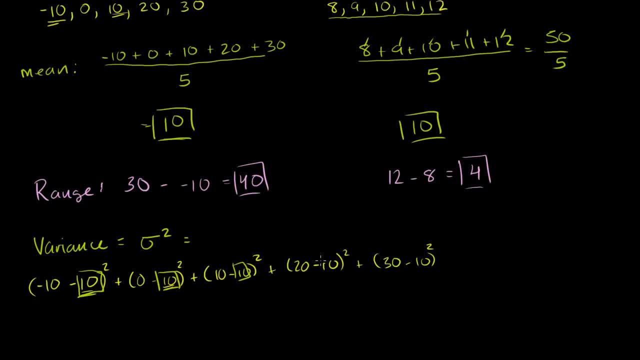 This is the mean, right there. That is the mean. I'm finding the difference between every data point and the mean, squaring them, summing them up and then dividing by that number of data points. I'm taking the average of these numbers, of the. 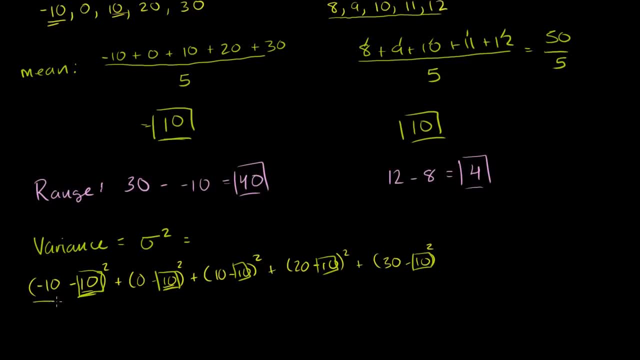 squared distances. So when you say it kind of verbally it sounds very complicated. but you're just taking each number. What's the difference between that, the mean square? it Take the average of those. So I have 1,, 2,, 3,, 4, 5.. 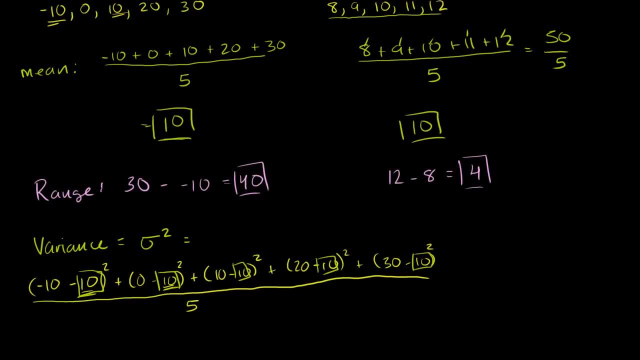 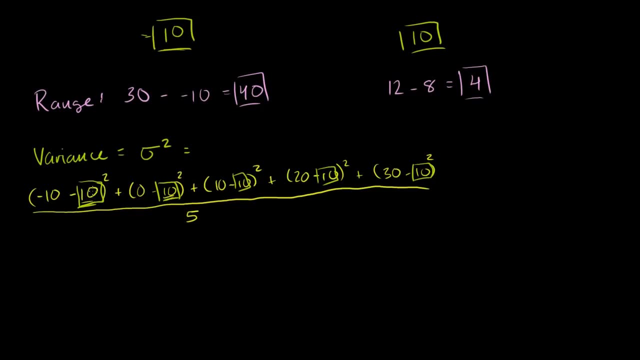 Divide by 5.. So what is this going to be equal to Negative? 10 minus 10 is negative 20.. Negative 20 squared is 400.. 0 minus 10 is negative. 10 squared is 100.. So plus 100.. 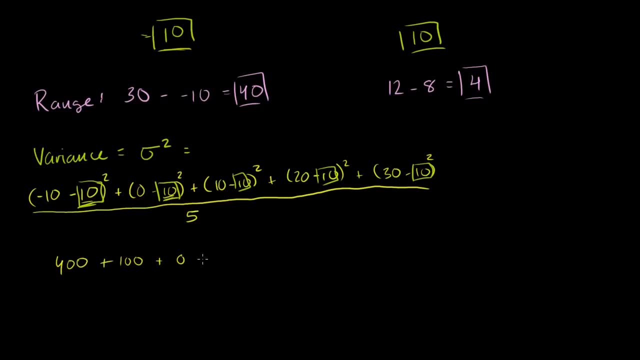 10 minus 10 squared, That's just 0 squared, which is 0.. Plus 20 minus 10 is 10, squared is 100.. Plus 30 minus 10,, which is 20, squared, is 400.. All of that over 5.. 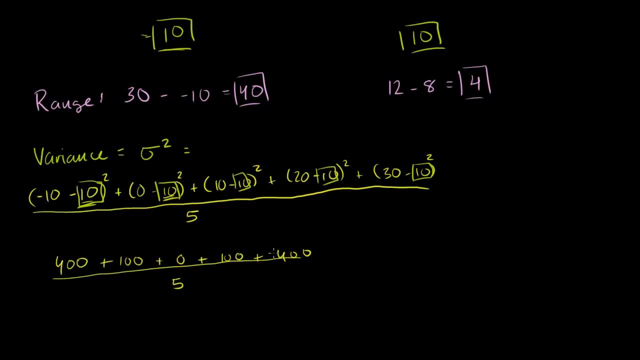 And what do we have here? 400 plus 100.. Plus 100 is 500. Plus another 500 is 1,000.. It's equal to 1,000 over 5, which is equal to 200.. So in this situation, our variance is going to be 200. 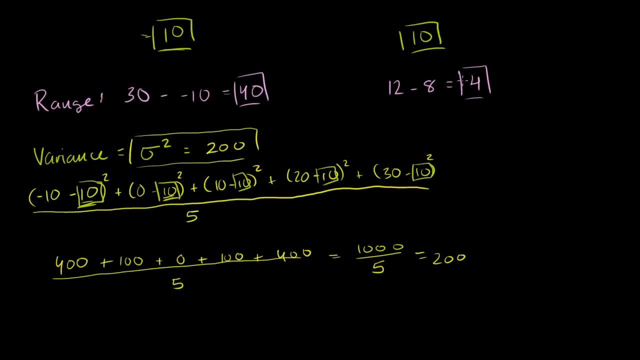 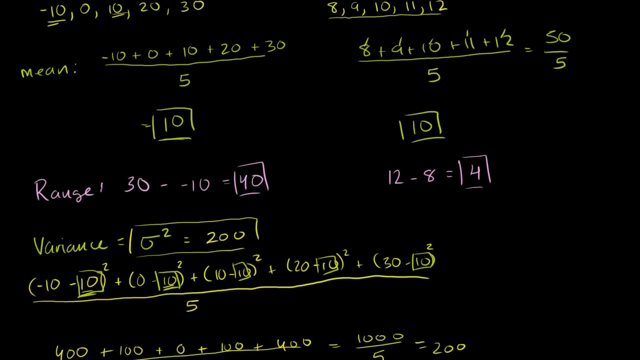 That's our measure of dispersion there, And let's compare it to this data set over here. Let's compare it to the variance of this less dispersed data set. Let me scroll over a little bit So we have some real estate, although I'm running out. 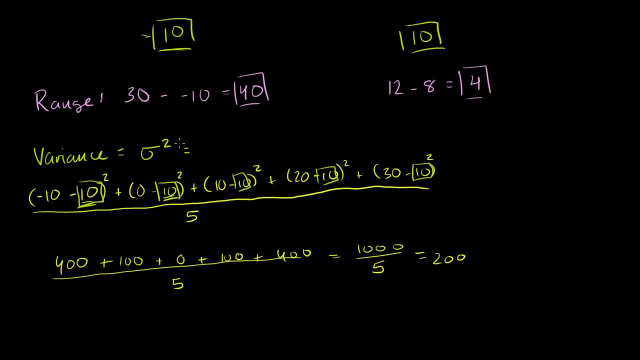 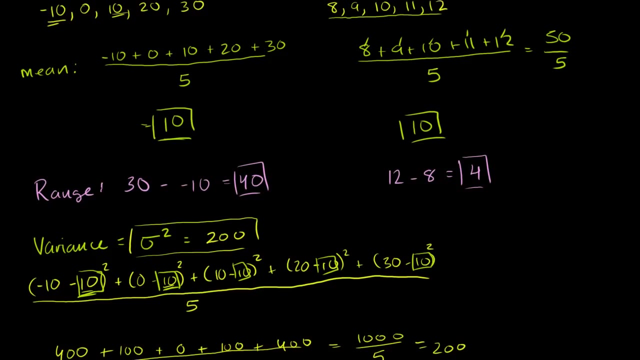 So in this situation our variance is going to be 200.. That's our measure of dispersion there And let's compare it to this data set over here. Let's compare it to the variance of this less dispersed data set. Let me scroll over a little bit. 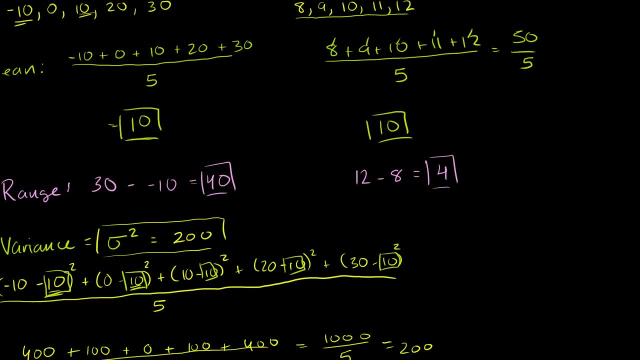 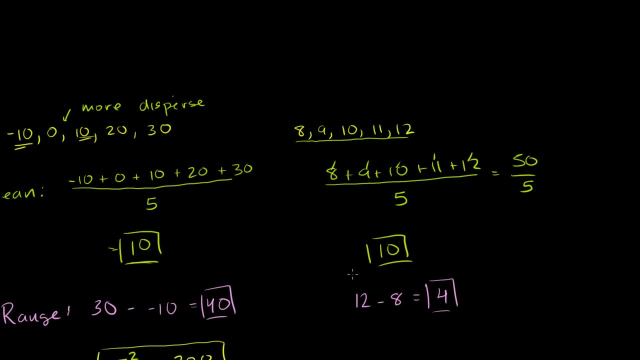 OK, So we have some real estate. although I'm running out, Maybe I could scroll up here. There you go. So let me calculate the variance of this data set. So we already know its mean. So its variance of this data set is going to be equal to. 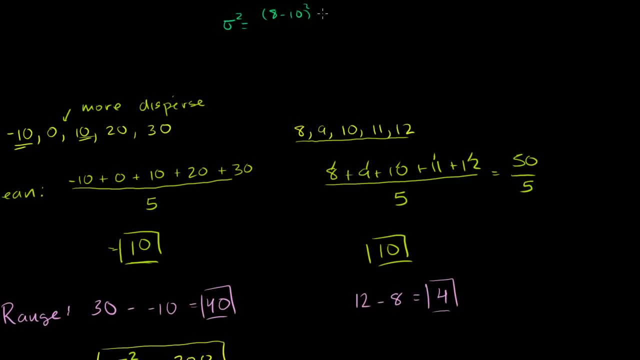 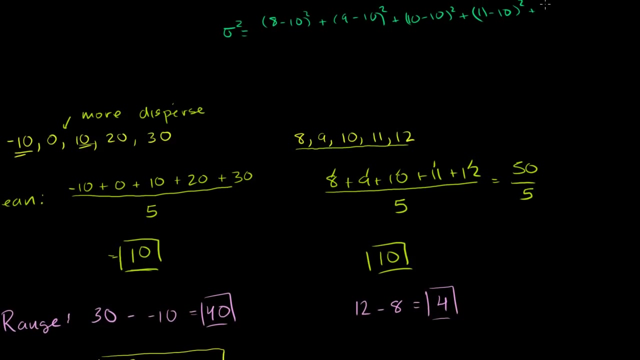 8 minus 10 squared plus 9 minus 10 squared plus 10 minus 10 squared plus 11 minus 10.. Let me scroll up a little bit: Squared plus 12 minus 10 squared. Remember that 10 is just the mean that we calculated. 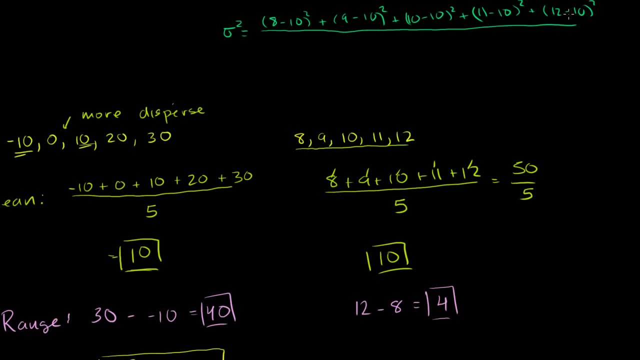 You have to calculate the mean first Divided by we have 1,, 2,, 3,, 4, 5 squared differences. So this is going to be equal to: 8 minus 10 is negative, 2 squared is positive 4.. 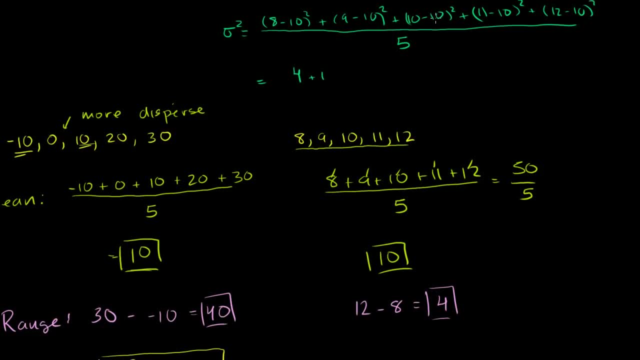 9 minus 10 is negative. 1 squared is positive. 1. 10 minus 10 is 0 squared, You still get 0.. 1. 11 minus 10 is 1.. Square it, you get 1.. 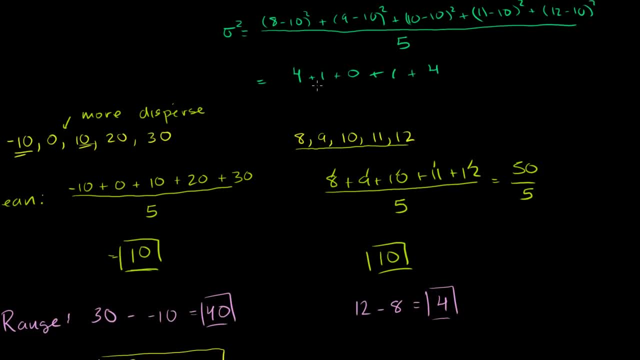 12 minus 10 is 2.. Square it, you get 4.. And what is this? equal to? All of that over 5.. This is 10 over 5.. So this is going to be 10 over 5, which is equal to 2.. 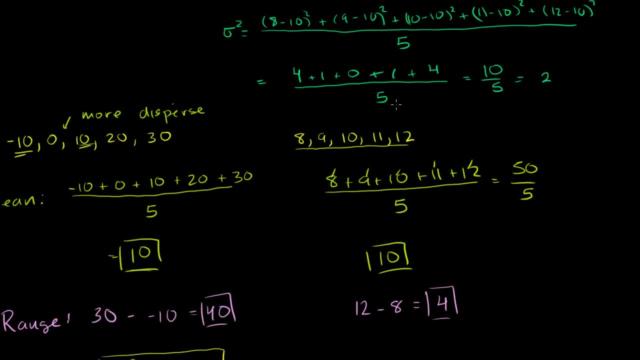 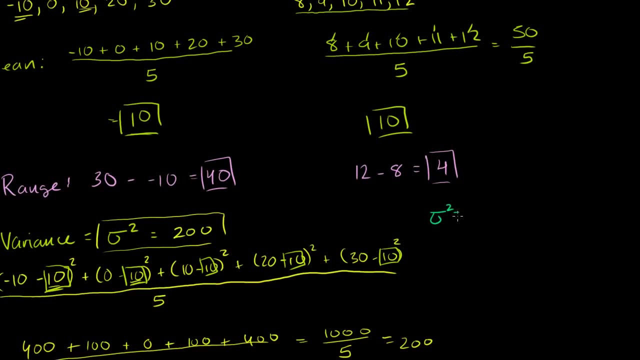 So the variance here- let me make sure I got that right- Yes, we have 10 over 5.. So the variance of this less dispersed data set is a lot smaller. the variance here, The variance of this data set right here, is: 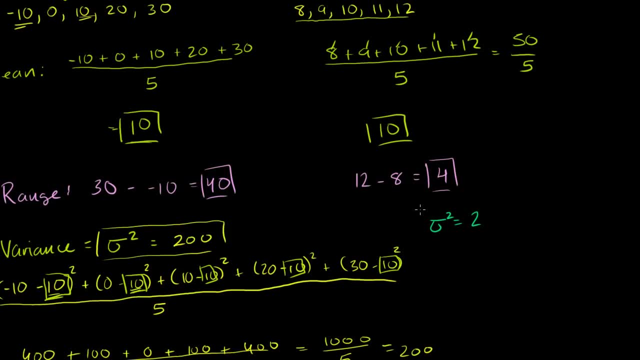 only 2.. So that gave you a sense. That tells you: look, this is definitely a less dispersed data set than that there. Now the problem with the variance is you're taking these numbers, you're taking the difference between them and the mean, then you're squaring it. 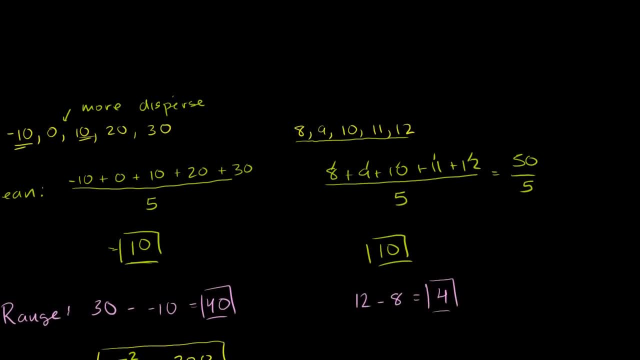 Maybe I could scroll up here. There you go. So let me calculate the variance of this data set. So we already know its mean. So its variance of this data set is going to be equal to 8 minus 10 squared plus 9 minus 10 squared plus 10 minus. 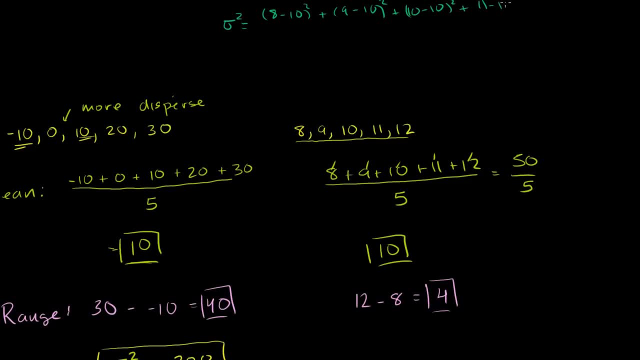 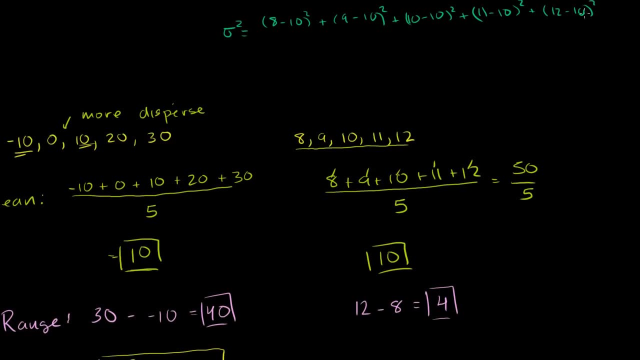 10 squared plus 11 minus 10.. Let me scroll up a little bit: Squared plus 12 minus 10 squared. Remember that 10 is just the mean that we calculated. You have to calculate the mean first Divided by. we have 1,, 2,, 3, 4, 5 squared differences. 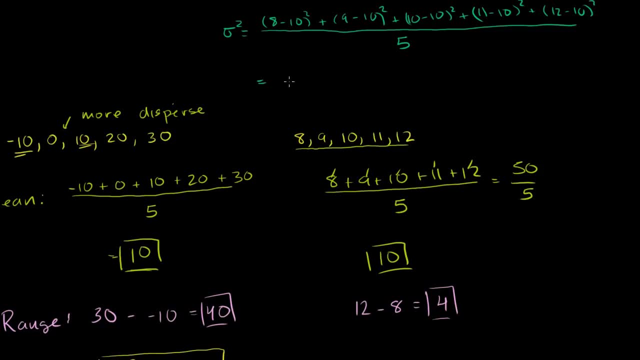 So this is going to be equal to: 8 minus 10 is negative. 2 squared is positive. 4.. 9 minus 10 is negative. 1 squared is positive. 1.. 10 minus 10 is 0 squared. You still get 0.. 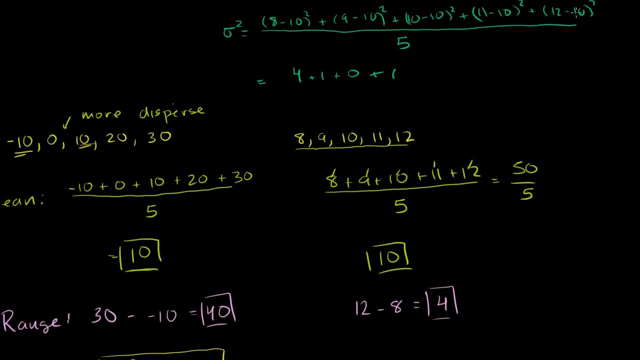 11 minus 10 is 1 squared, You get 1.. 12 minus 10 is 2 squared, You get 4.. And what is this? equal to All of that over 5.. This is 10 over 5.. 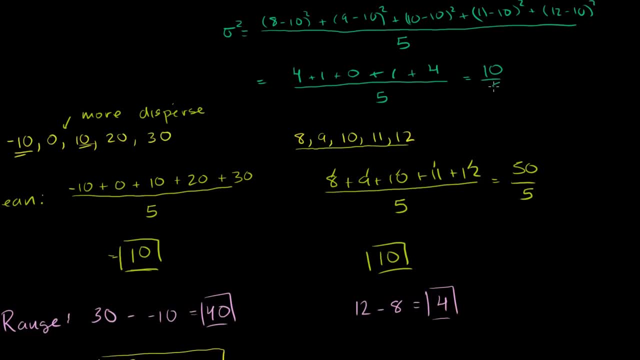 So this is going to be 10 over 5, which is equal to 2.. So the variance here- let me make sure I got that right- Yes, we have 10 over 5.. So the variance of this less dispersed data set is a lot. 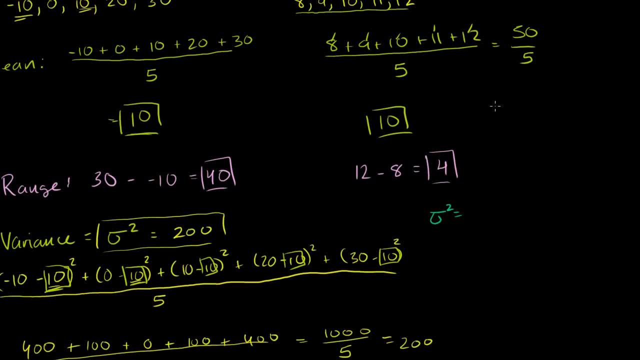 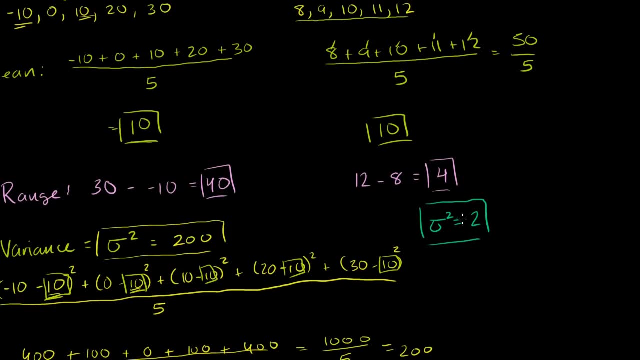 smaller the variance here. The variance of this data set right here is only 2.. So that gave you a sense. That tells you: look, this is definitely a less dispersed data set than that there. Now the problem with the variance is you're taking 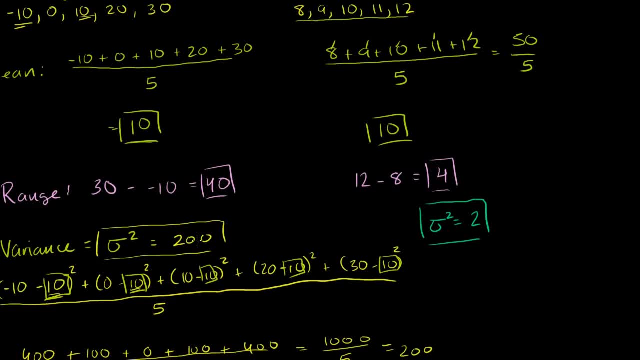 these numbers, you're taking the difference between them and the mean, then you're squaring it. It kind of gives you a bit of an arbitrary number. And if you're dealing with units, let's say if these are each negative, well, let's say they're distances. 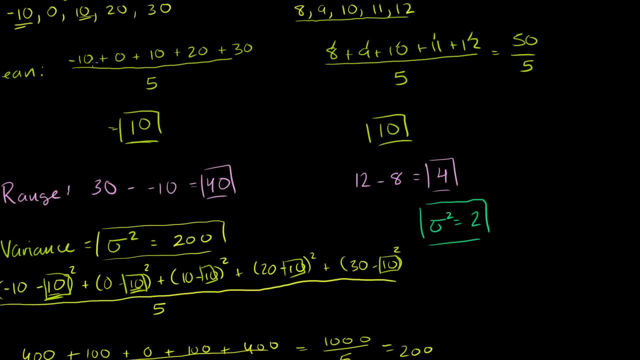 It kind of gives you a bit of an arbitrary number And if you're dealing with units, let's say if these are each negative, well, let's say they're distances, So this is negative. 10 meters. 0 meters, 10 meters, this is. 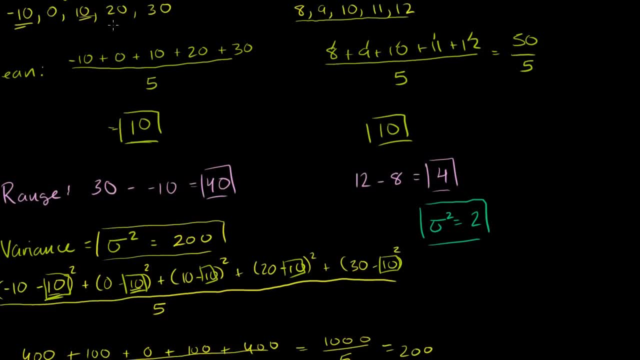 So this is negative: 10 meters, 0 meters, 10 meters, This is 8 meters, so on and so forth. Then when you square it, you get your variance in terms of meters squared. It's kind of an odd set of units. 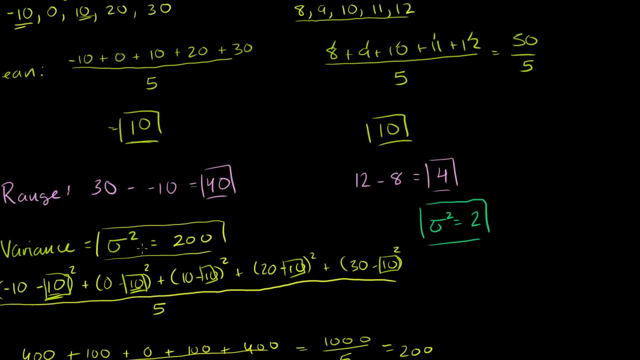 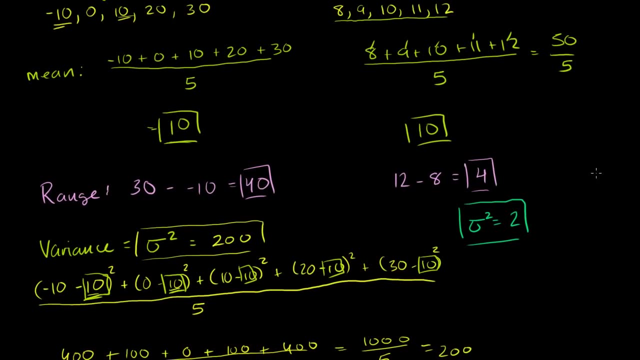 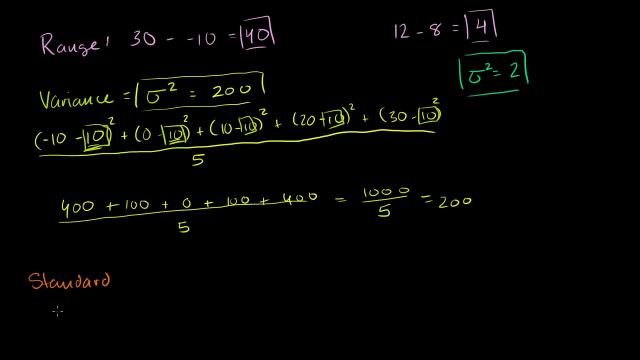 8 meters, so on and so forth. Then when you square it, you get your variance in terms of meters squared. It's kind of an odd set of units. So what people like to do is talk in terms of standard deviation, which is just the square root of the variance. 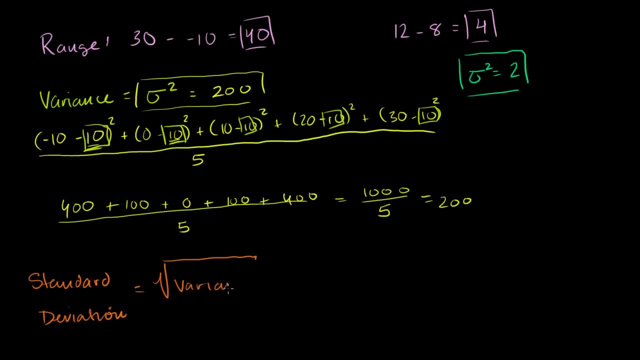 It's just the square root of the variance or the square root of sigma squared, And the symbol for the standard deviation is just sigma. So now that we've figured out the variance, it's very easy to figure out the standard deviation of both of these characters. 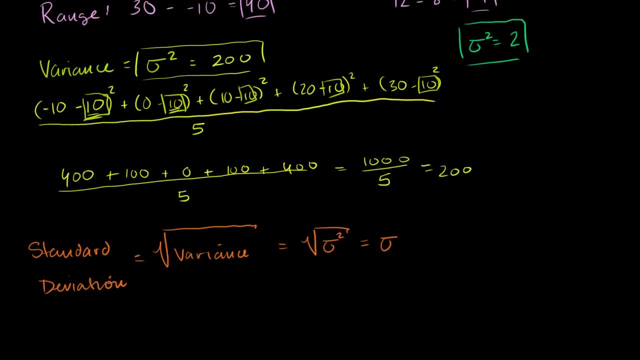 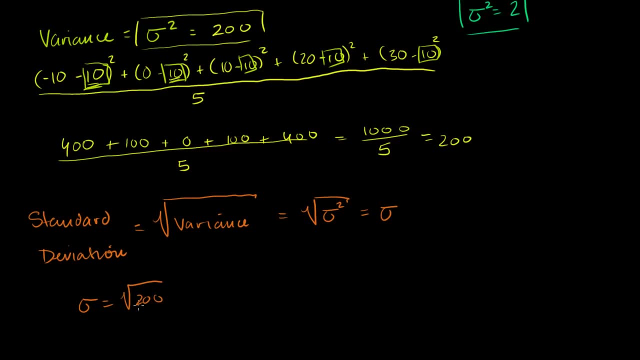 The standard deviation of this first one up here, of this first data set, is going to be the square root of 200.. Square root of 200 is what The square root of 2 times 100. This is equal to 10 square roots of 2.. 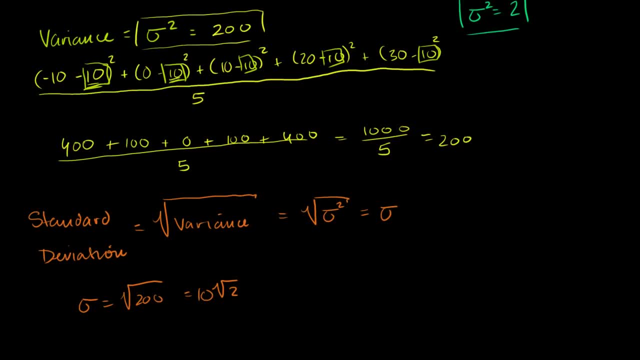 That's that first data set. Now the variance of the second data set is just going to be the square root of 2.. The variance is going to be the square root of that. Sorry, the standard deviation of the second data set is: 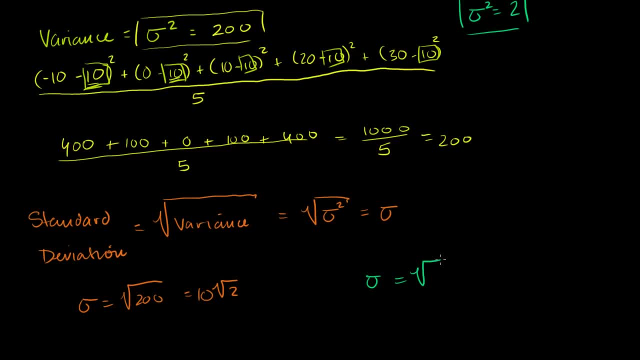 going to be the square root of its variance, which is 2, which is just 2.. So the second data set has 1 tenth the standard deviation as this first data set. This is 10 roots of 2.. This is just the root of 2.. 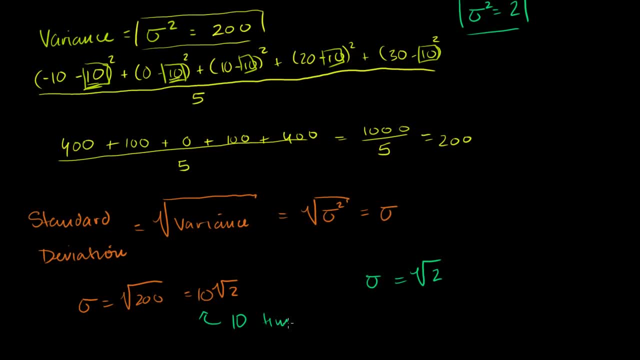 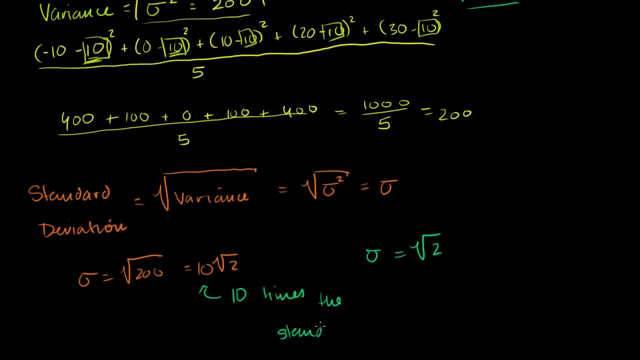 So this is 10 times the standard deviation And this, hopefully, will make a little bit more sense. Let's think about it. This has 10 times more of the standard deviation than this, And let's remember how we calculated it. 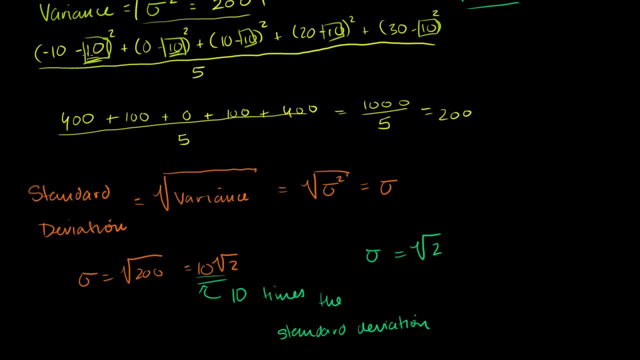 Variance. we just took each data point: how far is it away from the mean squared that took the average of those. Then we took the square root, really just to make the units look nice. But the end result is we said that that first data set has. 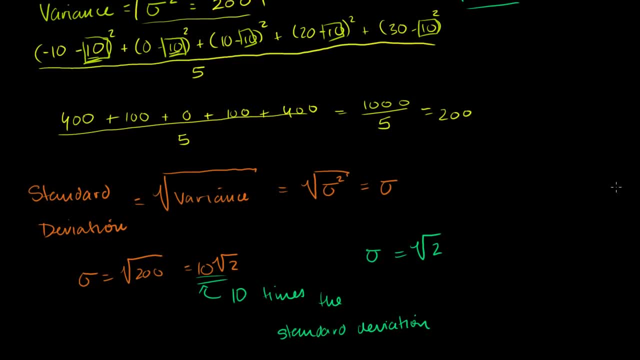 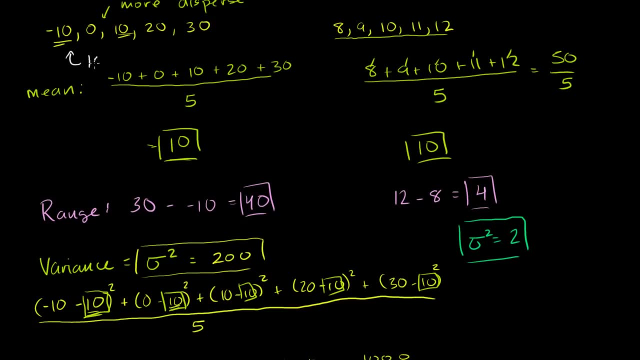 10 times the standard deviation as the second data set. So let's look at the two data sets. This has 10 times the standard deviation, which makes sense intuitively, right? I mean they both have a 10 in here. 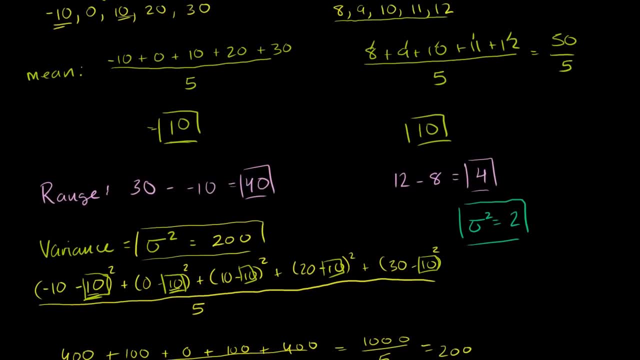 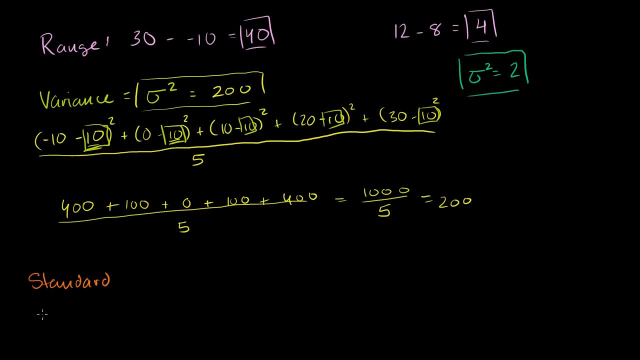 So what people like to do is talk in terms of standard deviation, Which is just the square root of the variance. It's just the square root of the variance, Or the square root of sigma squared, And the symbol for the standard deviation is just sigma. 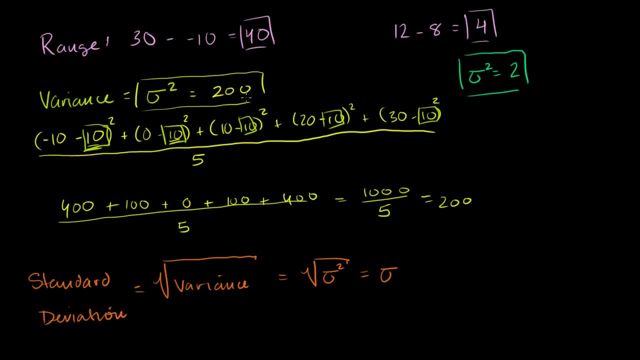 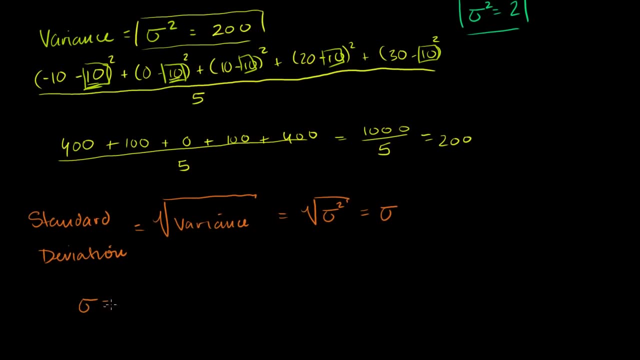 So now that we've figured out the variance, it's very easy to figure out the standard deviation of both of these characters. The standard deviation of this first one up here, of this first data set, is going to be the square root of 200.. 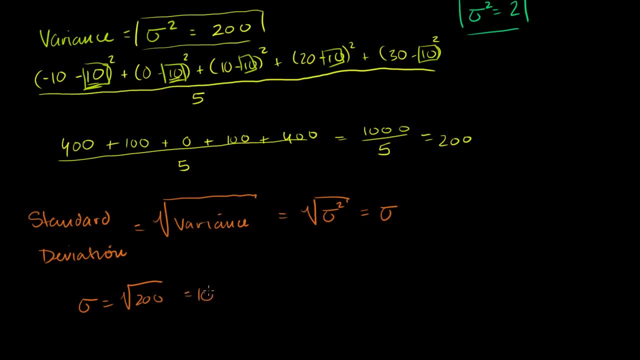 Square root of 200 is what The square root of 2 times 100.. This is equal to 10 square roots of 2.. That's that first data set. Now the variance of the second data set is just going to be the square root of 2.. 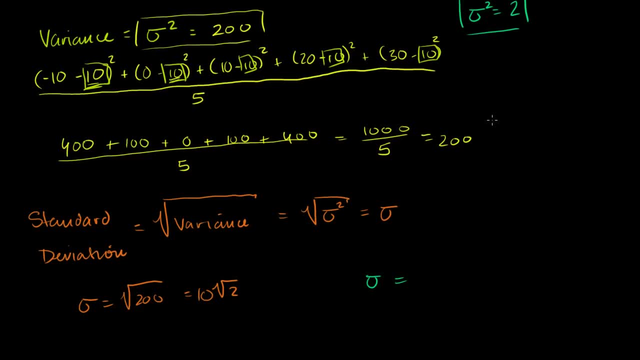 Variance of the second data set is just going to be the square root of 2.. Variance is going to be the square root of that. Sorry, The standard deviation of the second data set is going to be the square root of its variance, which is 2.. 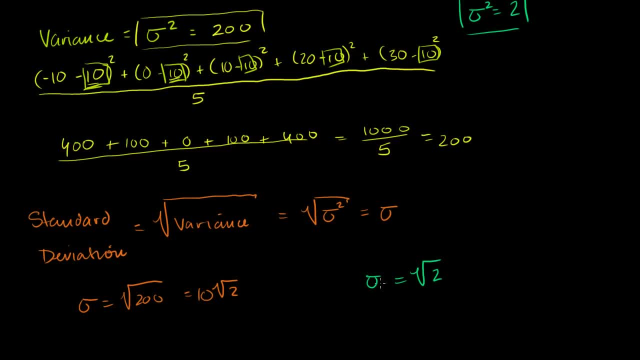 Which is just 2.. So the second data set has 1 tenth the standard deviation as this first data set. This is 10 roots of 2.. This is just the root of 2.. So this is 10 times the standard deviation. 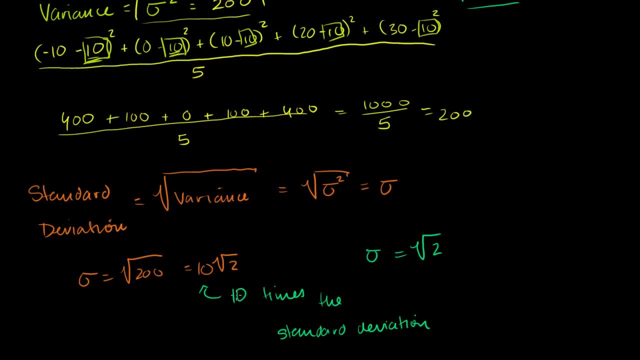 And this, hopefully, will make a little bit more sense. Let's think about it. This has 10 times more of the standard deviation than this, And let's remember how we calculated it: Variance, we just took each data point. how far is it away? 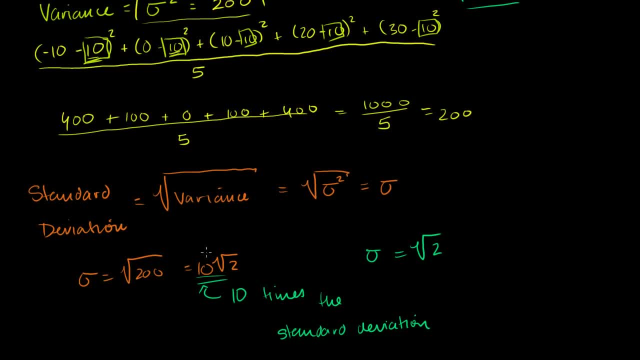 from the mean squared. that took the average of those. Then we took the square root, really just to make the units look nice. But the end result is we said that that first data set has 10 times the standard deviation as the second data set. 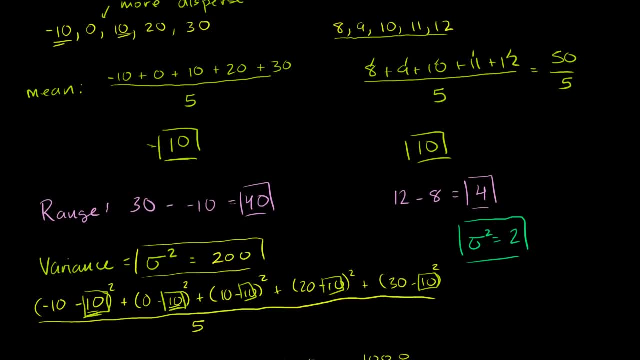 So let's look at the two data sets. This has 10 times the standard deviation, which makes sense intuitively, right? I mean they both have a 10 in here, But each of these guys 9 is only 1 away from the 10.. 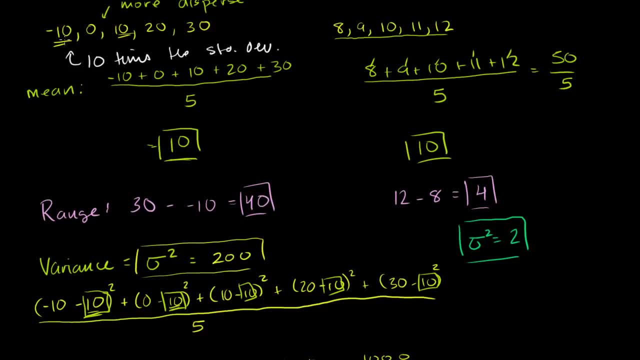 0 is 10 away from the 10, 10 less 8 is only 2 away. This guy's 20 away, So it's 10 times on average further away. So the standard deviation, at least in my sense, is giving. 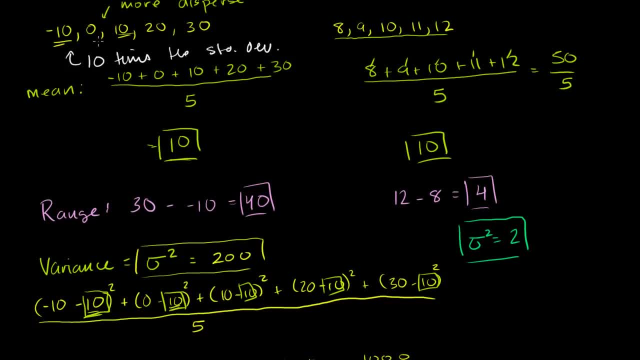 But each of these guys- 9- is only 1 away from the 10.. 0 is 10 away from the 10,. 10 less 8 is only 2 away. This guy's 20 away. So it's 10 times on average further away. 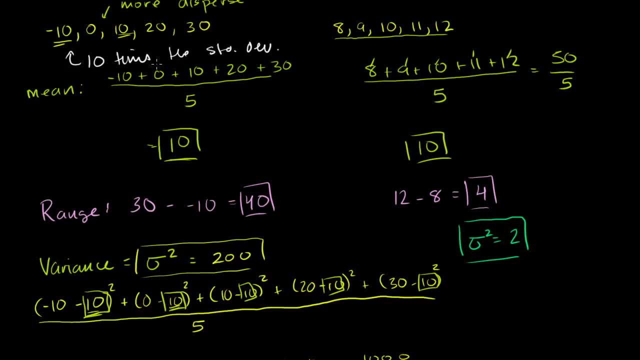 So the standard deviation, at least in my sense, is giving a much better sense of how far away, on average, we are from the mean. Anyway, hopefully you found that useful. 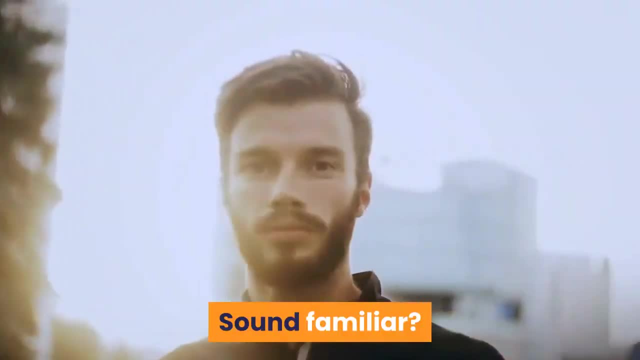 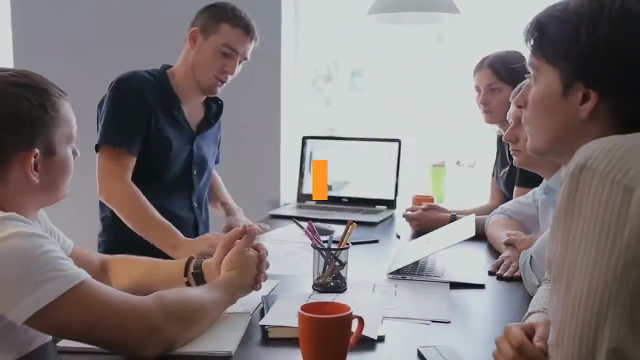 Do a great job and you get a prize. Sound familiar. This approach to behavioral management is used everywhere for adults and children, whether at home or at school, in the workplace or in the gym, When it's used consistently and in a structured manner for children with special 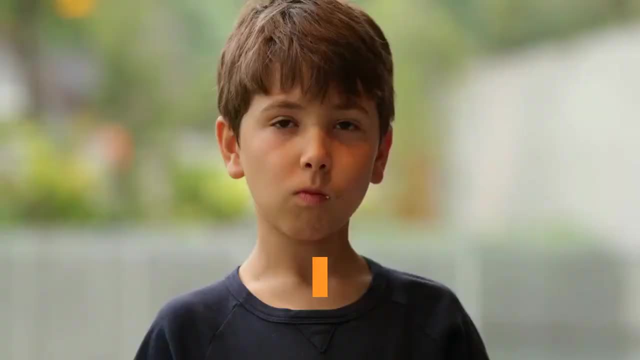 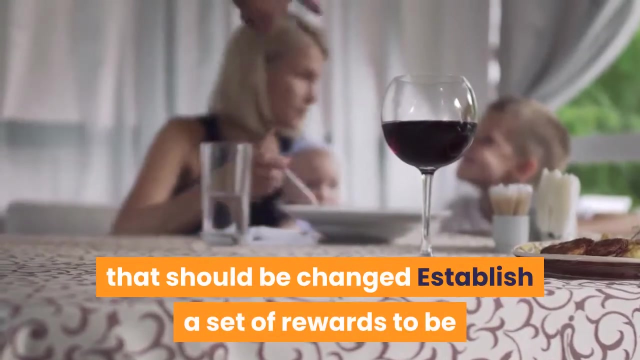 needs. it is often called behavior management. Behavior management is really just as simple as it sounds. Identify the problem, behaviors that should be changed. establish a set of rewards to be earned for good behavior. stick to the plan most of the time. Behavior management systems. 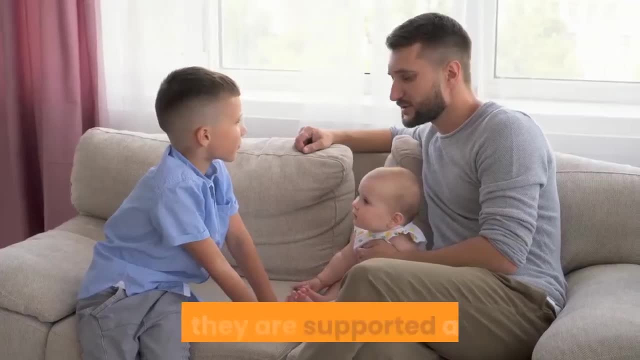 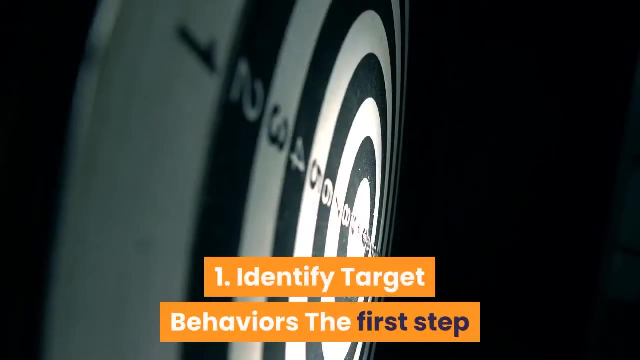 are set up by specialists in a school setting. Ideally they are supported at home so that children receive the same messages in different situations. 1. Identify target behaviors. The first step is to identify the behaviors you want to see and the behaviors you want to decrease or 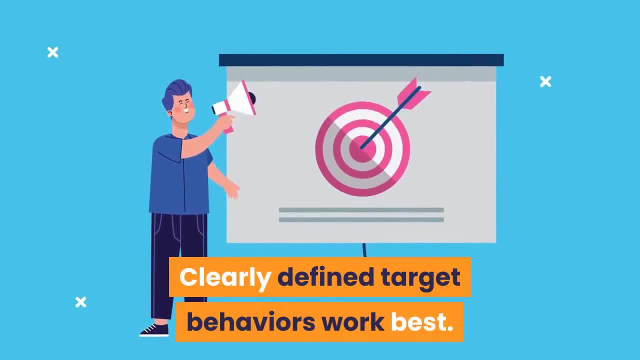 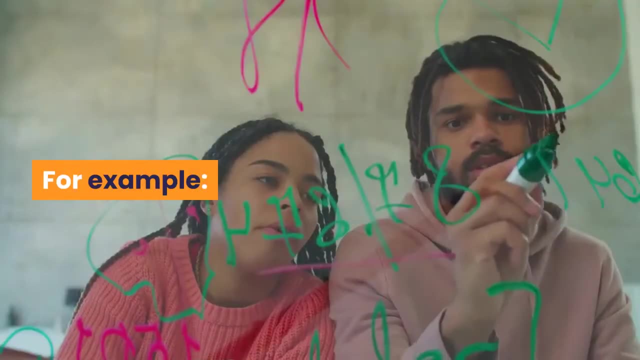 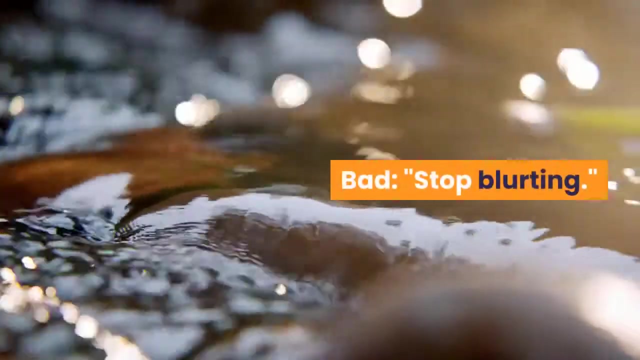 eliminate. Clearly defined target behaviors work best. Ideally, the behaviors should be concrete, measurable and easy To identify. for example: good, raise your hand rather than blurting out answers in math class today. Bad, stop blurting. 2. Identify effective rewards. Rewards need to be motivating to be.